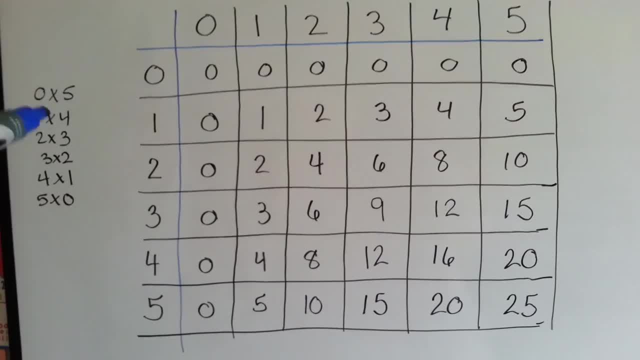 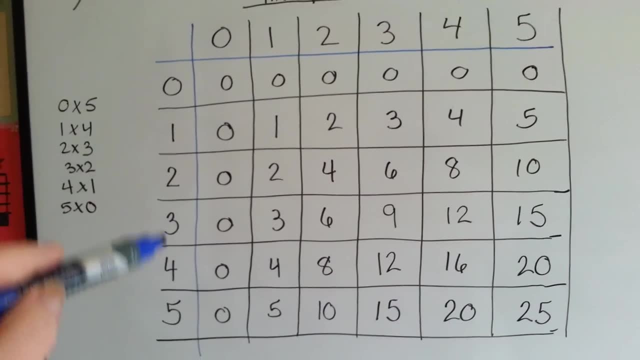 Believe it or not, we can find some patterns in here. Let's do these and see what happens. This is the first number and then that's the second factor. So 0 times 5 would be 0 times 5.. 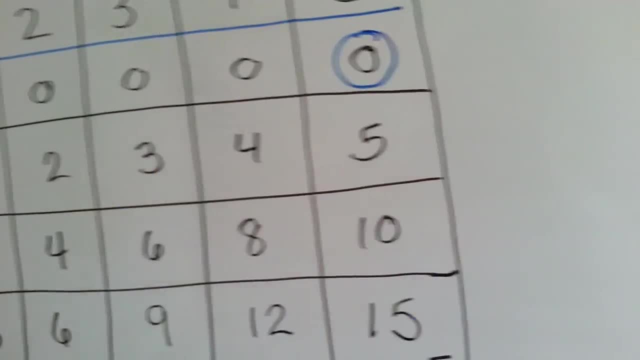 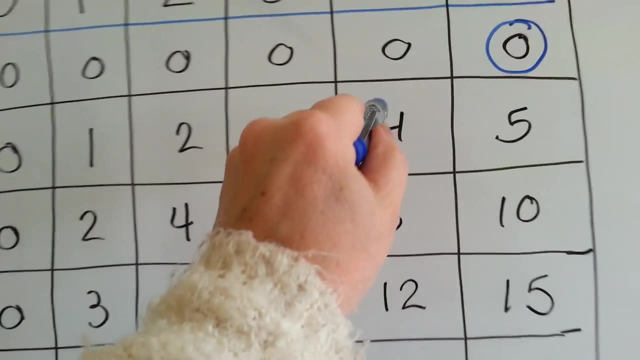 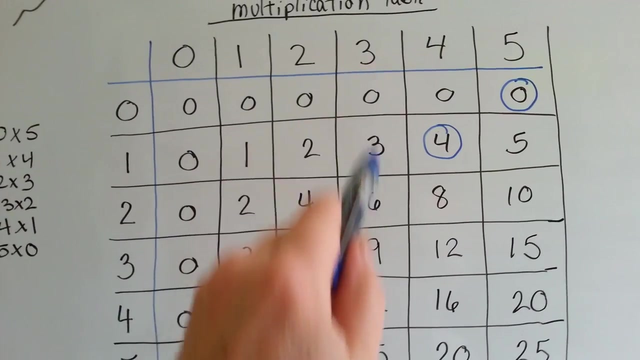 So that puts us here: Alright, 1 times 4.. 1 times 4.. The next one is 2 times 3.. 2 times 3.. Do you see the pattern that's happening? Can you already tell what's going to happen? 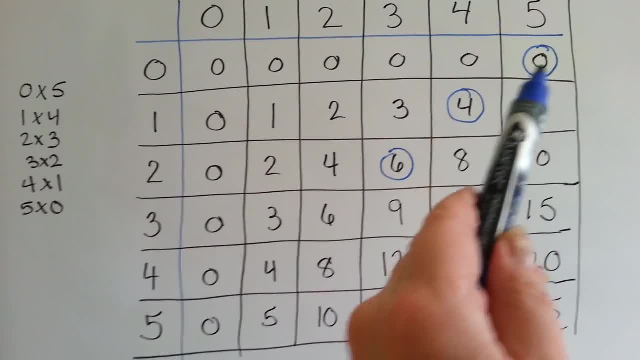 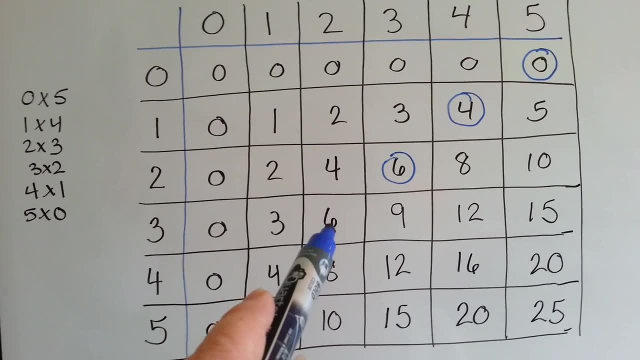 What number do you think is going to be the next one? I circle Just from what you see is happening. can you tell what the pattern is that I'm making? The next one is 3 times 2.. 3 times 2.. I bet you knew I was already going to do that one. 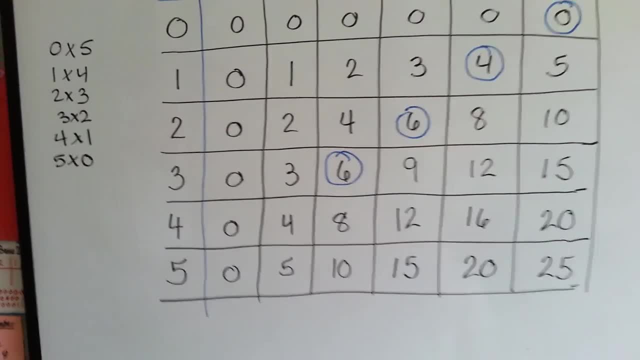 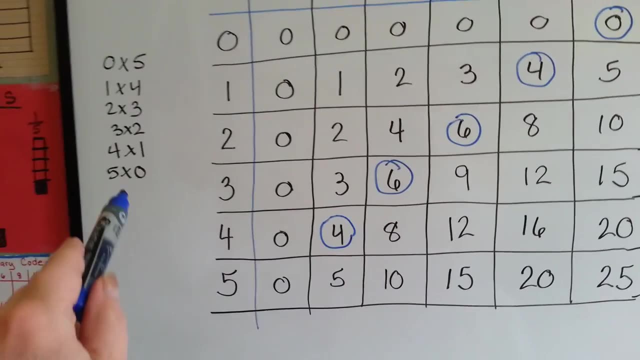 didn't you? The next one is 4 times 1, and I bet you know where that is, don't you? 4 times 1, and then we have 5 times 0.. Do you see the pattern we made? 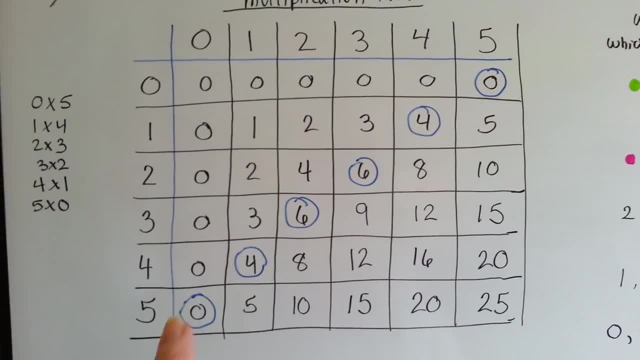 Not only did we make a visual pattern of it angling downward like this, but we made a number pattern saying 0, 4, 6, 6, 4, 0.. 0, 4, 6, 6, 4, 0.. 0, 4, 6, 6, 4, 0.. 0, 4, 6, 6, 6, 4, 0.. 0, 4, 6, 6, 6, 4, 0.. 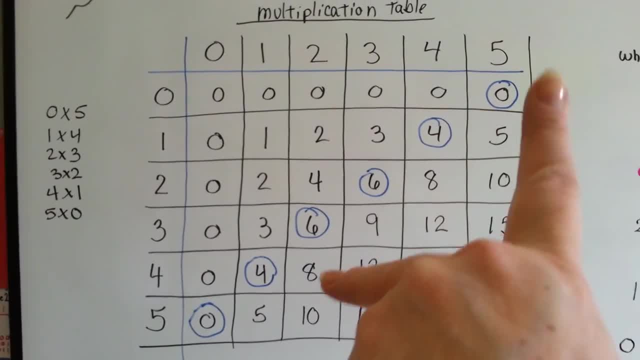 0, 4, 6, 6, 6, 0. There's two 6's in the middle, then two 4's and then zero's on the end. See that We made a pattern. You can make all kinds of patterns with the multiplication table. 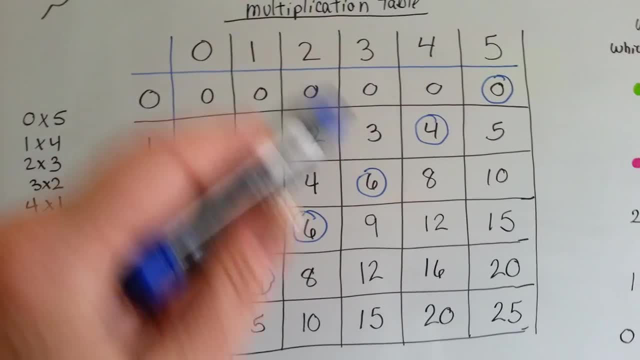 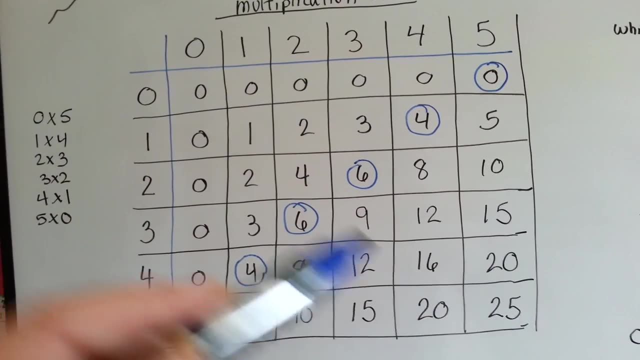 You should try it. You should get a blank sheet of paper, make the multiplication tables on it and see what kind of patterns you could make. Did you know that you can count by odd numbers going down in an angle and even numbers going? 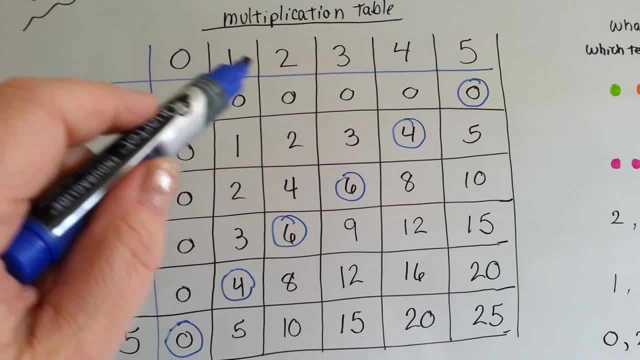 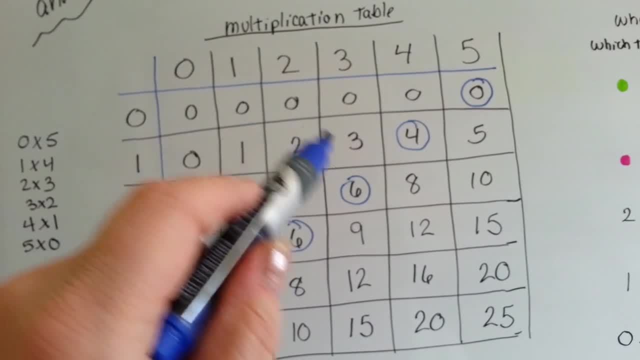 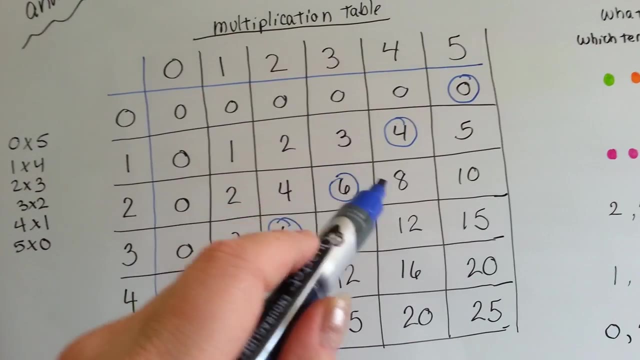 down by the 2's Yep. Look it: 0 and 3 is 3, right. 0 plus 3 is 3.. 3 plus what is 8? 5.. So 3, 5.. What would be the next odd number? 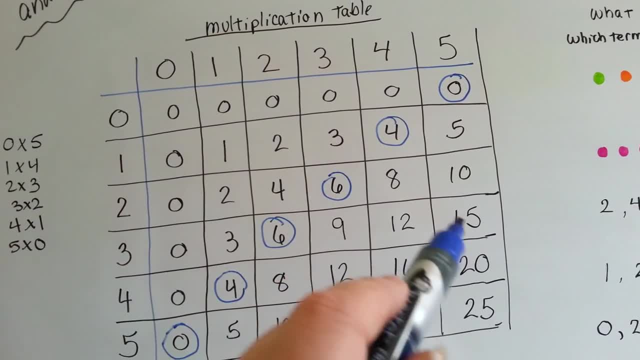 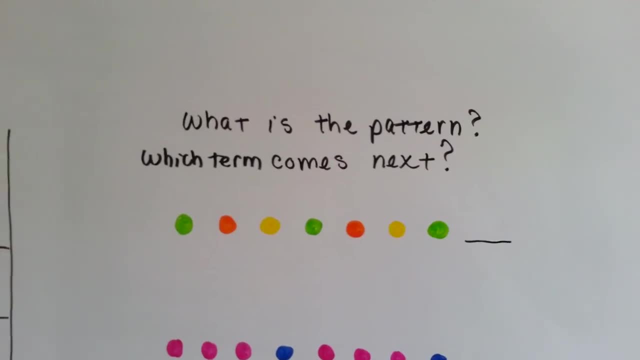 7.. 8 plus 7 is 15.. So do you see how I add the next odd number? and it's coming down, isn't it? So, knowing that, what do you think comes next? What's the next term in this pattern? 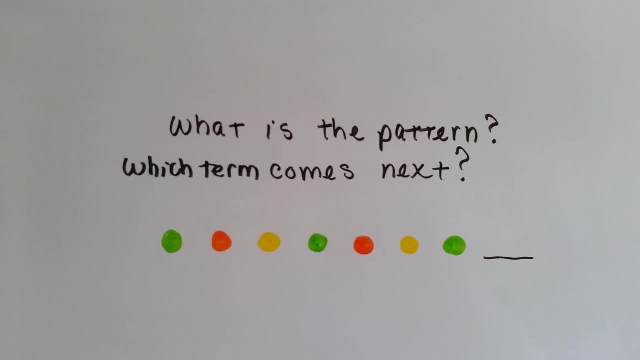 Can you tell? Well, it's green circle, orange circle, yellow circle, green circle, orange circle, yellow circle, green circle. What do you think is next? What is the next term? Well, this one's not that hard. 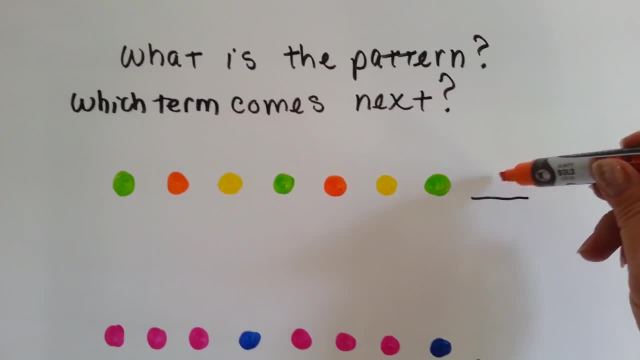 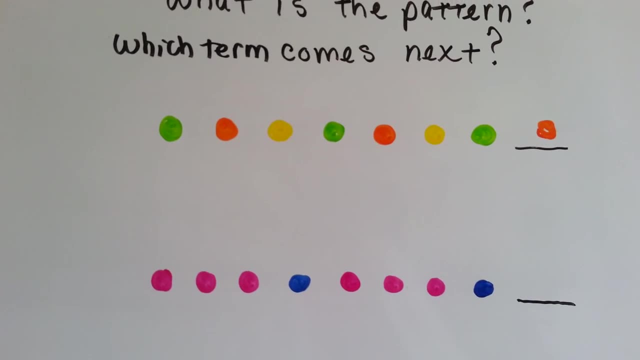 You should be able to get this one, okay. The next one should be an orange circle. okay, How about this one? Pink circle, pink circle, pink circle, blue circle, pink circle, pink circle, pink circle, blue circle. 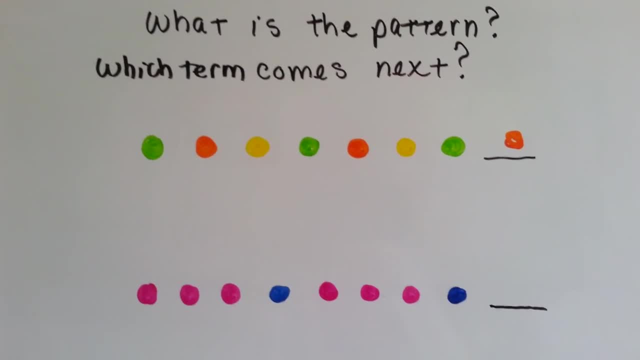 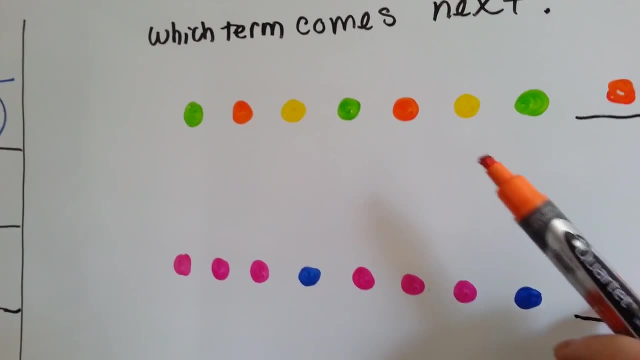 What's the very next one? If you said blue, that's a good generic term. If you said pink circle, you were right. Okay, better than fourth. OK, I will add that in here. All right, now let's look at these. 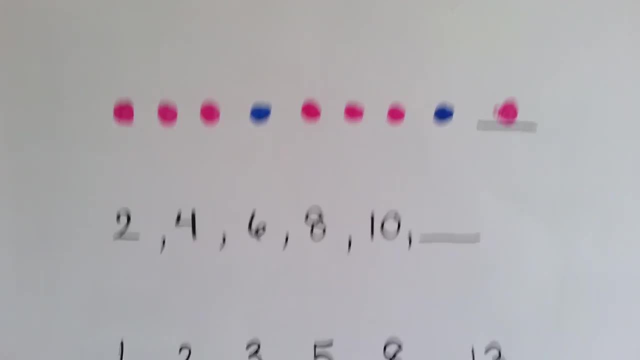 We've got number patterns. 6: educate pessoa say no, okay. What do you think is the next number for this one? 2 and then 4 and then 6 and then 8 and then 10.. What do you think goes here? Well, if you saw that they were skip counting by 2,, If you셔 that they were skip counting by 2,, 2 and then 4, and then 6, and then 8, and then 10,, what do you think goes here? 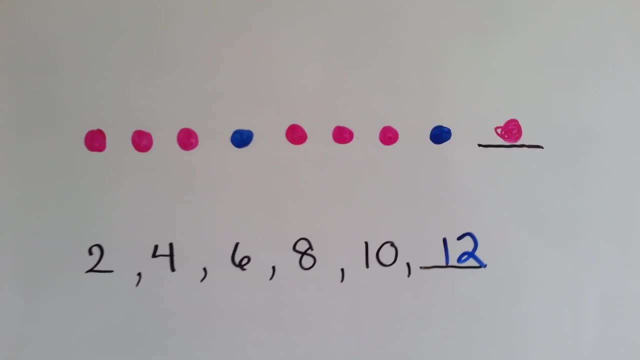 and that the next one is 12,. you're right. How about this one? What is the next term in this pattern? This one's a little harder. Can you figure out what the pattern is? It goes 1,, 2,, 3,, 5,, 8,, 13.. What is it doing? Well, if you look closely, 1 plus 2 is 3.. 2 plus 3 is 5. 3. 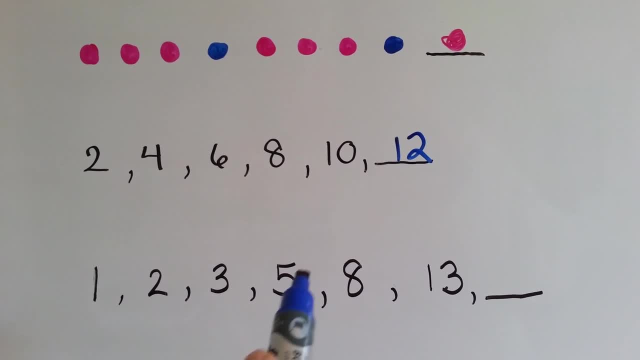 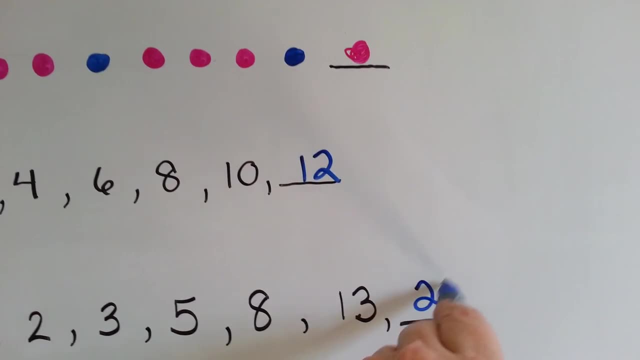 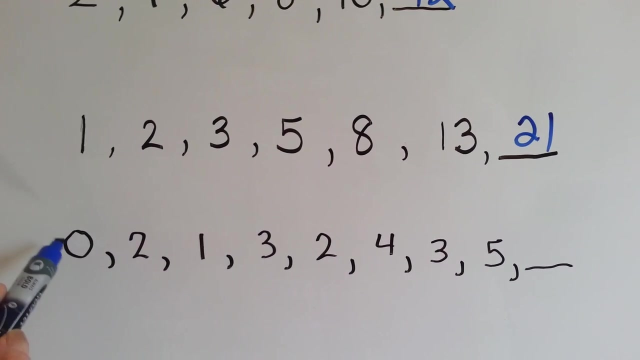 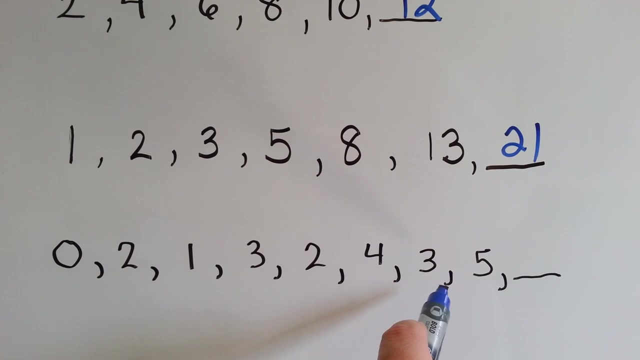 plus 5 is 8.. 5 plus 8 is 13.. So 13 plus 8 is, if you said, 21,. you were right. How about this one? Can you figure out the pattern to this one? This one's a little harder: 2, 1, 3, 2, 4, 3, 5, blank. 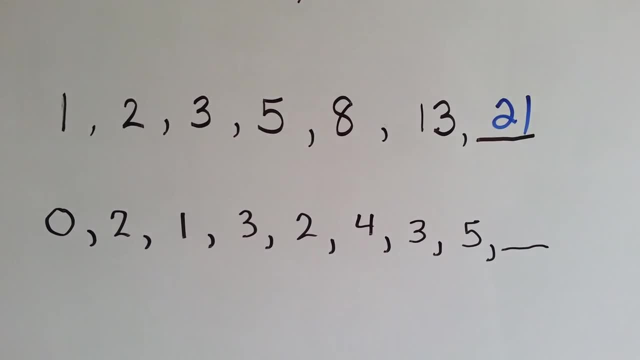 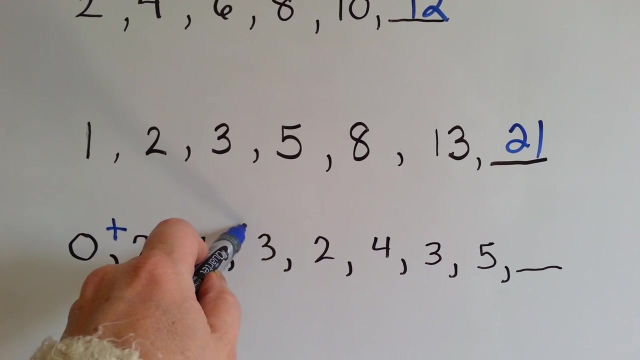 Can you tell What the pattern is on this one? You could pause it if you want to, because I'm going to tell the answer. This one is adding 2, and then taking away 1.. And then adding 2, and then taking away 1.. 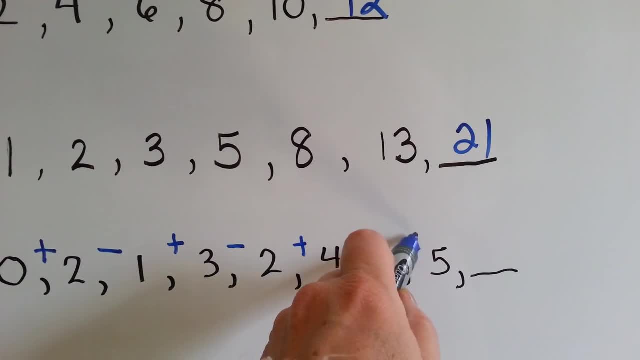 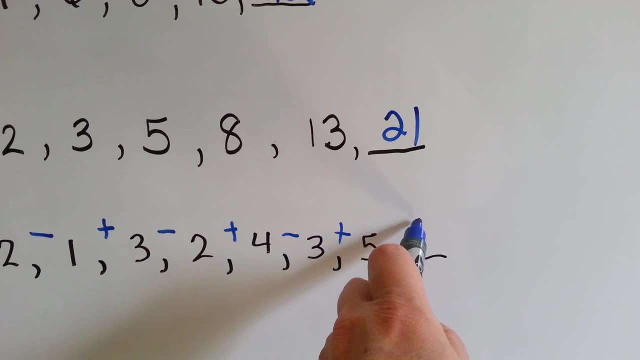 Adding 2, taking away 1, adding 2.. So if we took away 1, what would go here? 4.. If you said 4, you're right. Okay, they're getting a little harder. Can you figure out the? 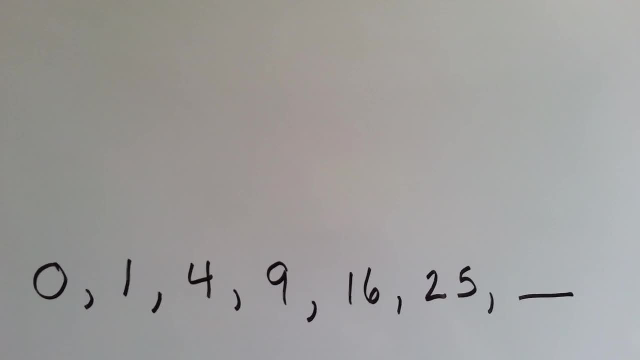 next term for this pattern? What's happening here? 0,, 1,, 4,, 9,, 16,, 25.. Hmm, If you want to pause the video so you can figure it out on your own, you should do it now, because I'm going to. 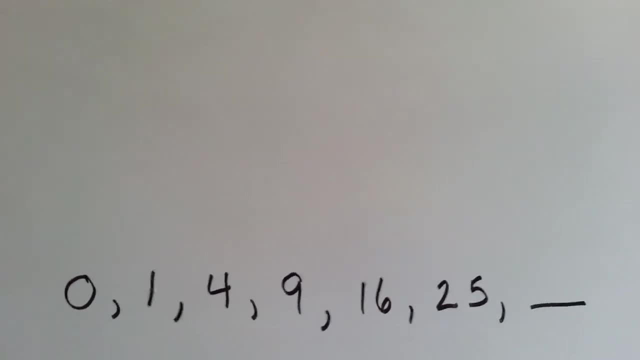 show you the answer. The numbers are going up by odd numbers. 1 and 0 is 1. 3. 1 and 3 is 4. 5. 4 and 5 is 9. 7. See, these are all the odd numbers. 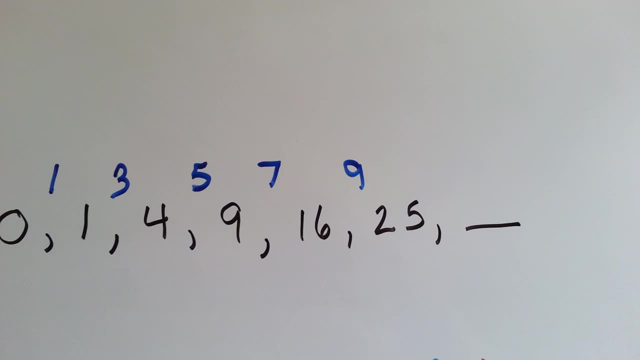 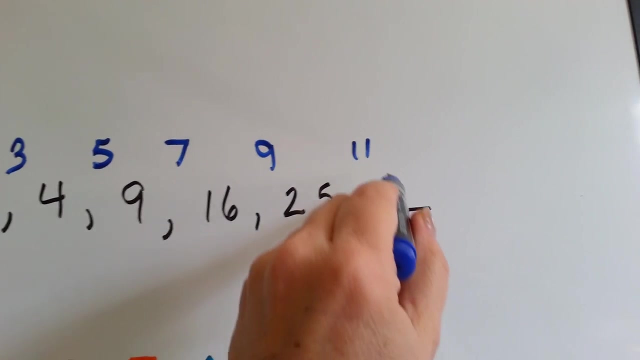 So what would come next after this? 16 and 9 is 25.. What would come here? What's the next odd number After 9.. 11.. So what number would come here If you said 36,? you're right, See. Okay, here's a colored. 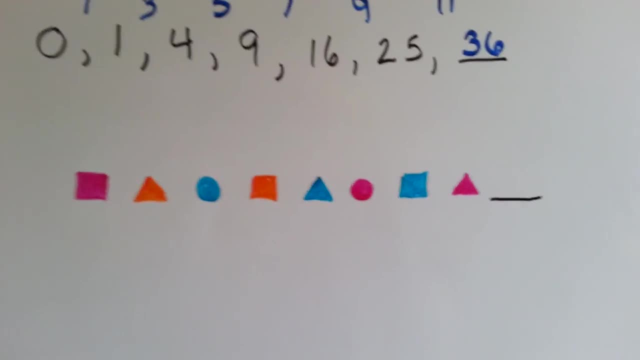 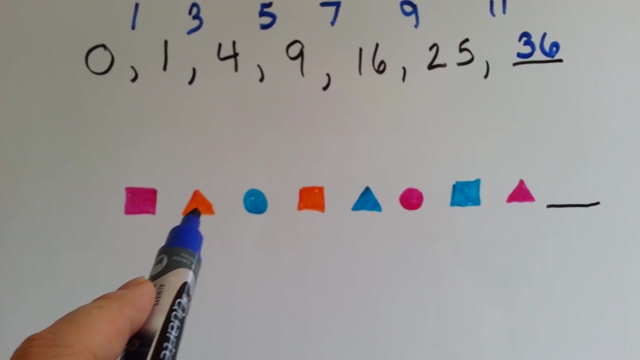 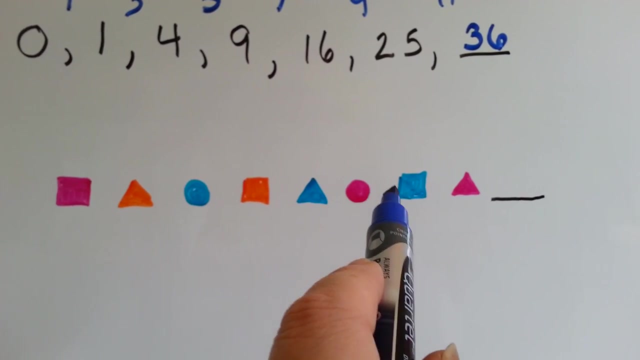 shaped pattern. See if you can figure this one out. This one's a little harder. We've got a pink square, an orange triangle and a teal ball. Then we've got an orange square and a, a teal triangle and a pink ball.